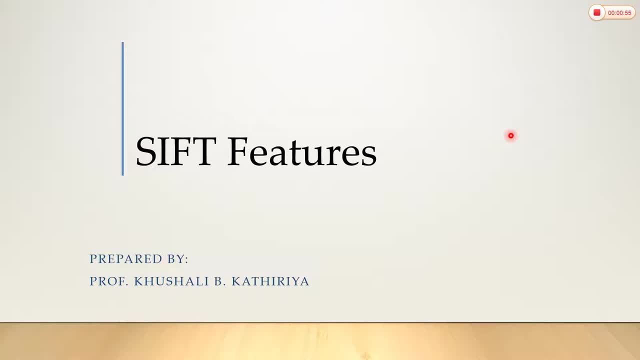 Like its curve shape, angle, Whatever it is, its ages point, What we call it? It is called features. So which feature is important? We will identify it using. So they have different kind of features, But here we have seen, we will have seen SIFT features. 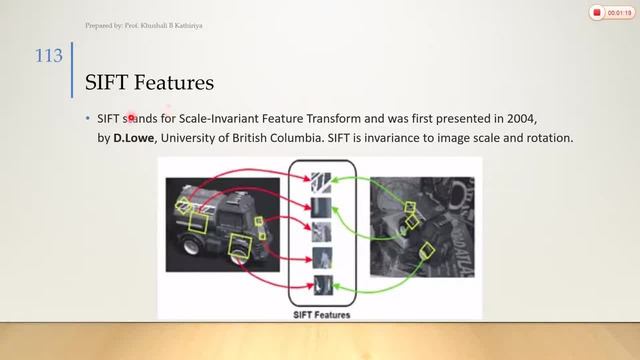 So, first of all, what is the SIFT features? SIFT features- that means SIFT stands for the scale. invariant features. transformation was the first present in 2004.. They are developed in 2004 with the LOG University of British Columbia. 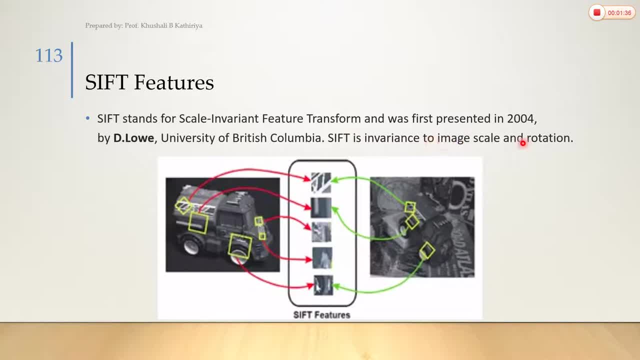 SIFT is the variance of image to image, scale and rotation. Okay, that means if we have to match two images, okay we have to check that. suppose we have one car and another car. We have to identify that. these two suppose that our Tata car and Suzuki car. 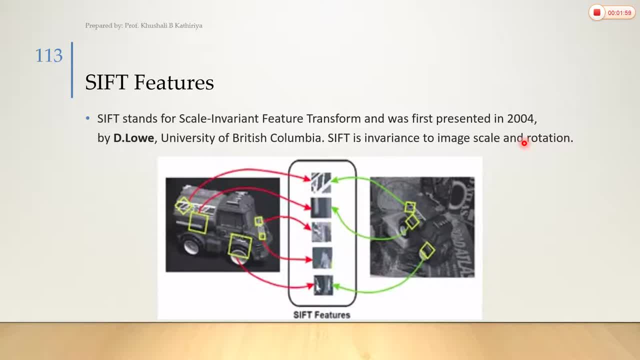 those two are the same. you know those two are different, but in the form of the image. how will the computer know if those two cars are the same or not? So what will it do? It will compare the features of different parts with that part with another image. 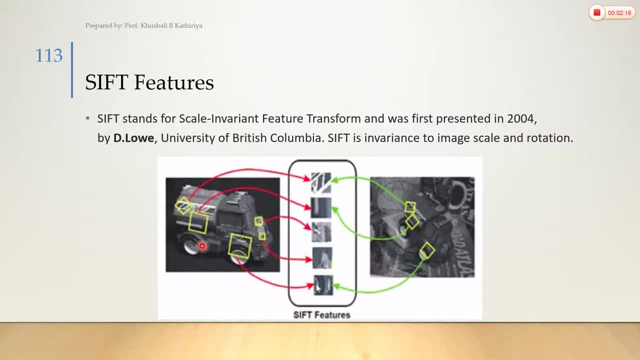 That means this is our one image and this is our second image Here. it has taken a portion. okay, it has zoomed this portion and identified its features, And those features are of some other image. So what will it do with that? It will match. 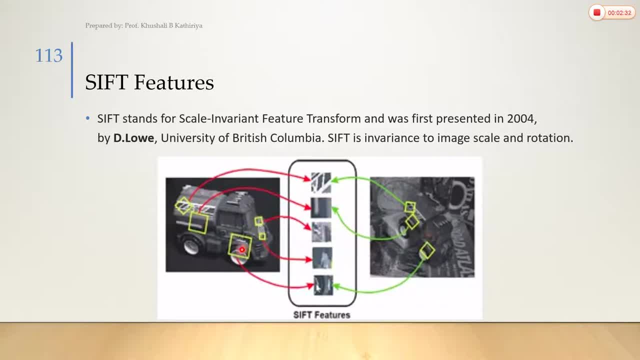 Same to same. this image will be compared with this. Okay, so this one is compared with this. one is compared with this. So here we don't know what kind of image it is. Okay, this is a small image. that means it is zoomed out from a distance, and this is a zoomed in image. 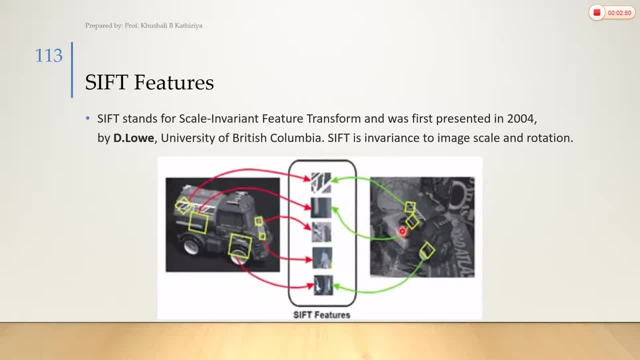 So we don't know. and its angle is also different. Okay, look here, there is a tire here, there is a tire here. according to that, this is its front, This is its side view, this is its front, This is its front. 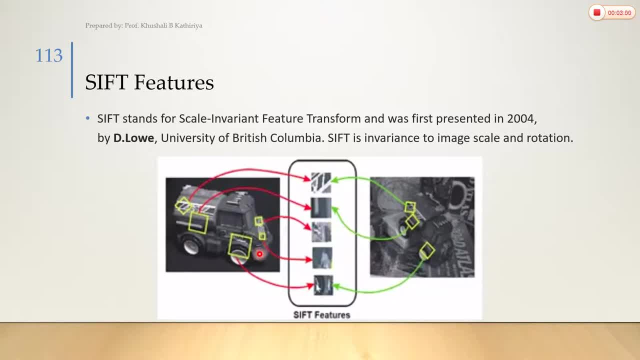 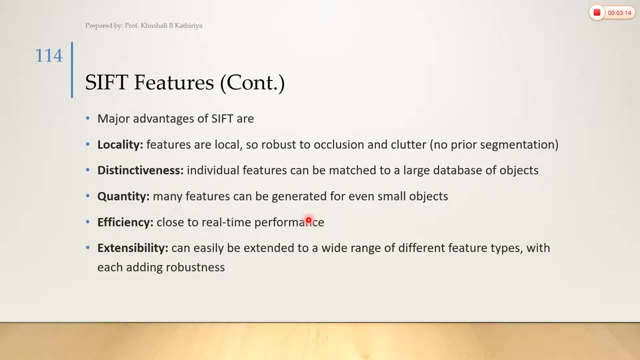 Still here we have SIFT features. that means the image that is being matched can be up to some limit, So these features are mostly used for image matching. So in this video we have discussed what is SIFT features, as well as application of SIFT features. 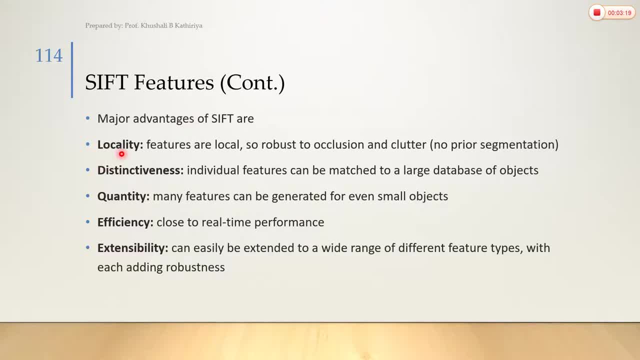 Okay. major advantage of SIFT are locality: Features are local, so robust to oculation and cluster. No prior segmentation. No need to segment the whole image into different kind of the part. Distractiveness: Individual features can be matched to a large database of objects. 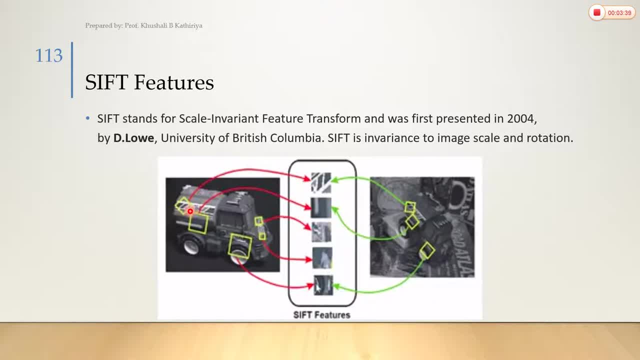 Here, what we have done is we have made a box of it, and what we have done is we have made a different kind of data set of individual features compared with another database object, And what we have done is we have compared another image with its object. 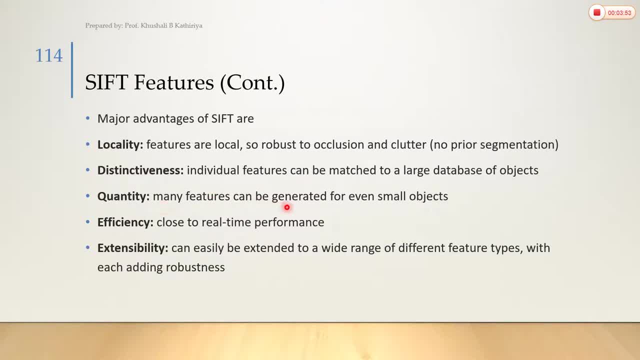 Quantity. Many features can be generated for even smaller objects. We have any small object Still we can generate multiple objects from it. Efficiency, Close to real-time performance and extensibility Can easily be extend to a wide range of different feature types, with each editing adding robustness. 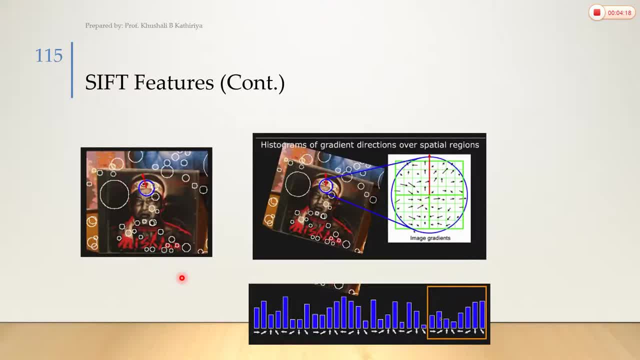 Okay, Now we see example of SIFT features. Suppose this is our image. Here I have done different kind of the circle. That means I have made a boundary, I have selected some shape, Okay. So first of all, if I can take rectangle like this, 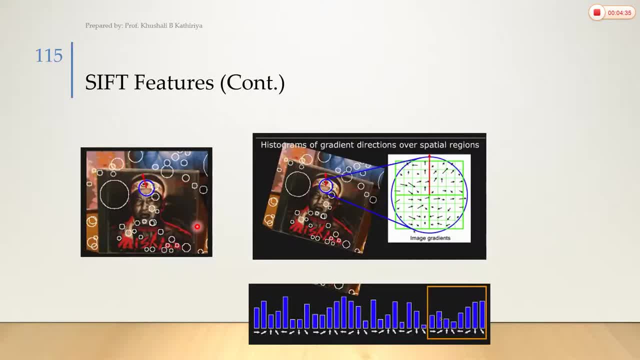 Or I can take triangle like this, Or I can take round or circle like this. Here what I have done is I have detected the area portion. Suppose I have detected something like this Here: blue line- Okay. 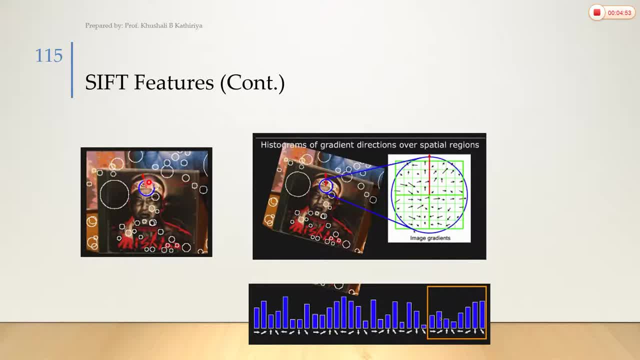 Maybe this image, That scaling That image, is not rotated, If we rotate it, Okay. So even after rotating the gradient of our image, The gradient we have learnt in HOG features, What will be the gradient? It will remain same. 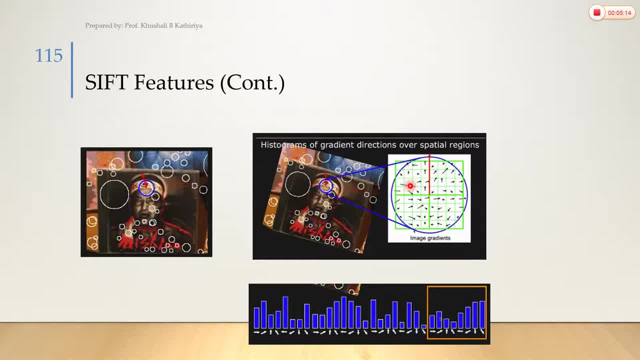 That means this angle, its attitude, magnitude and its direction. Okay, Its gradient direction. What we have done is we have located it here. If you don't know the gradient direction, Then you can watch the video of my HOG description. 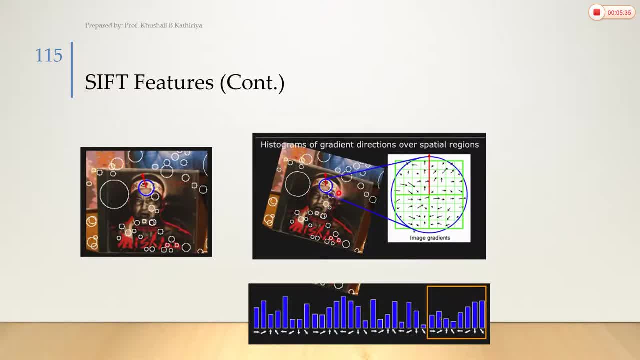 Okay, So this one is the SIFT features. What we have done is we have identified the gradient direction of this portion. We will compare this image and this image: The gradient direction of both the pixels And the features of those pixels. 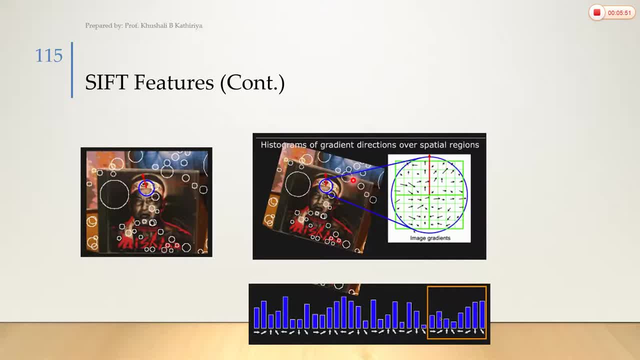 The important features. What we will do is we will compare them. Okay, After that, what we have done is we will plot the histogram of the magnitude, directed, gradient, direction. we have made. So, first of all, this portion, First is our quadrant. 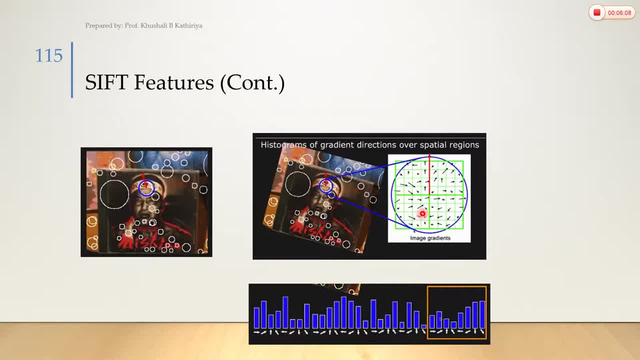 Okay, We have plotted its histogram till here. Second is the quadrant. We have defined its histogram again. Third is here And fourth is here, After that, the histogram of the entire circle. we have done is, we have merged it And we have normalized it. 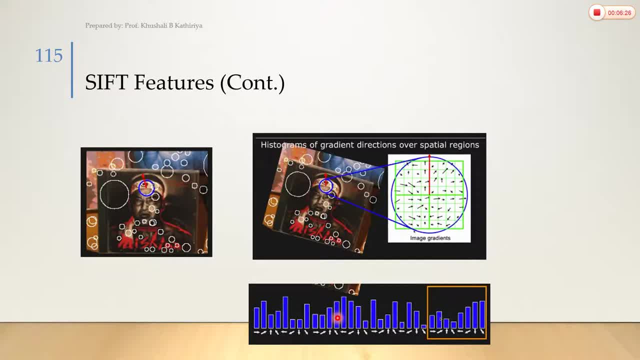 After normalizing it, we will get its feature set Particular for this area. By doing this, we have normalized the histogram of the entire image. Okay, Now what we have to do is this histogram If we want that. this portion is another image. 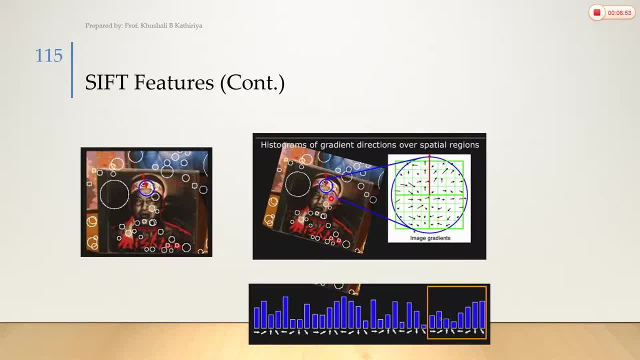 Suppose that another image is here. Suppose that another image is here. Suppose that another image is here. If we have to compare it with that, then how will we do it? So this is the comparison of our histogram. We will compare the area of the image of the same portion of the histogram of the other image. 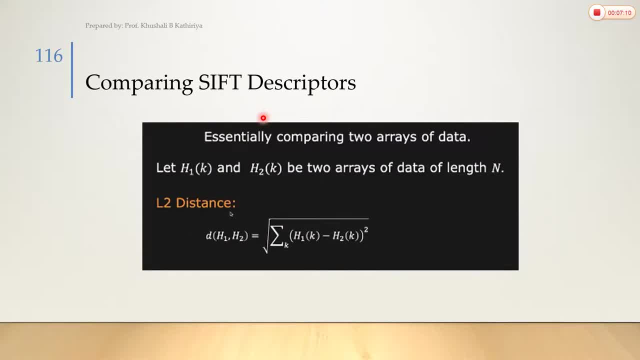 So how can we compare our SIFT descriptor? So the first method is L to distance. It is very simple. You can identify the distance between the two histograms. That means distance of H1 and distance of H2.. Okay, 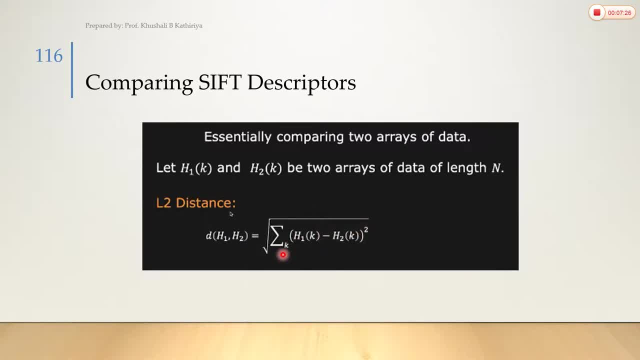 H1 minus H2, whole square And its summation. Whatever is the K value of our histogram? Okay, Energy value. What we have to do in that We have to identify its distance. That means distance between H1 and H2.. 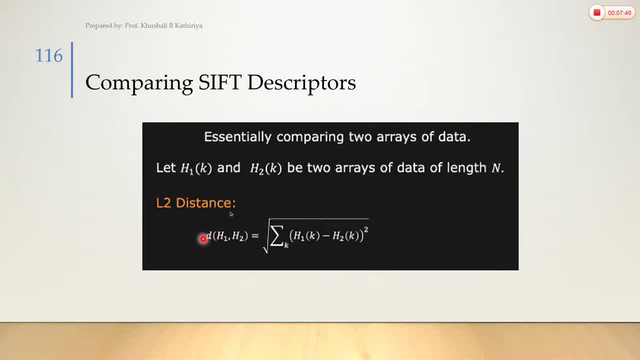 If your distance is 0.. Okay, This is the distance If it is 0.. So that means that your histogram is the shape of both the first image and the second image, And the features of both are same, So its histogram is the same of both. 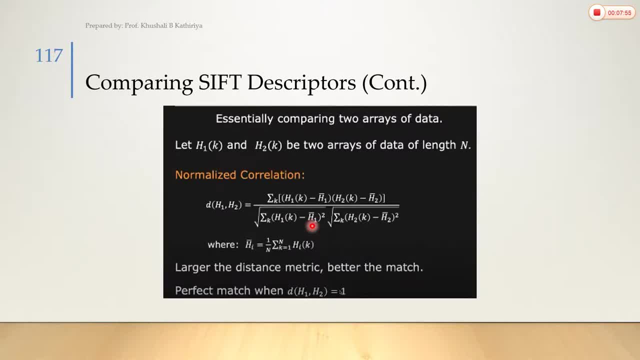 And its distance is 0.. Okay, Second method is the normalized correlation. What will happen in normalized correlation? We have to do summation with its bar value. That means H1 minus H1 bar value, H2 minus H2 bar value. 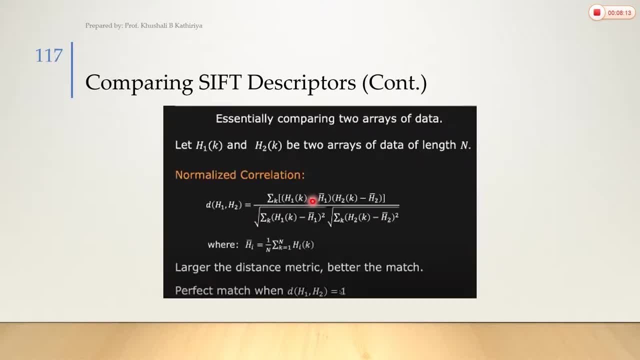 Upon its magnitude, Which we have identified: the distance value here, That is, H1 minus H bar And H2 minus H bar, The magnitude of these two, The magnitude of these two And, according to that, what we have to do. 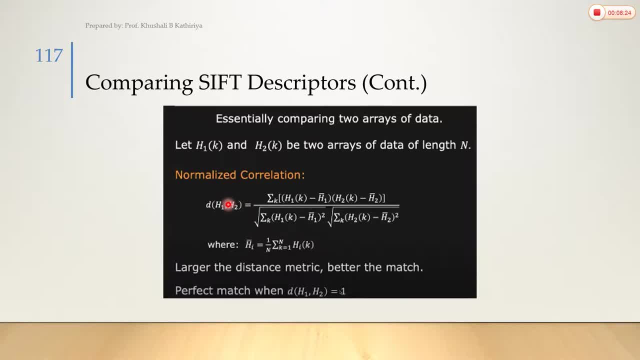 According to that, we have to identify its distance. If its distance here is 1.. D of 1., Okay, D is equal to 1.. Then our matches are perfect. That means our H1 and H2 histogram are same. 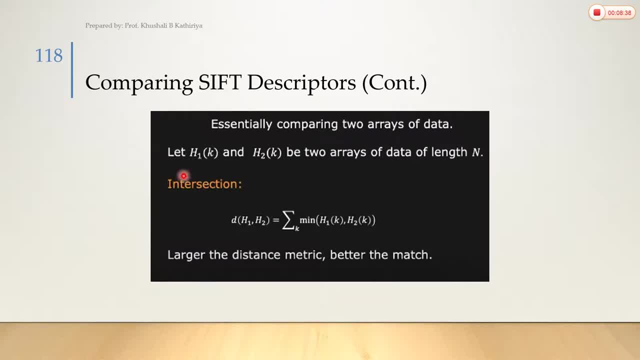 So our features are also same. And third one is the intersection. Intersection, that means minimum H1 of k and H2 of k. Larger the distance metric, better the match. What should come here, The minimum of which will come? What will be that? 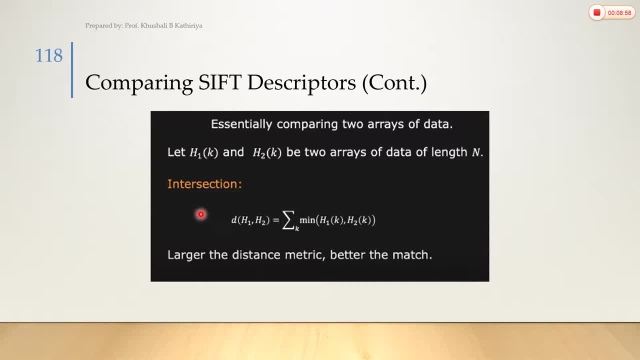 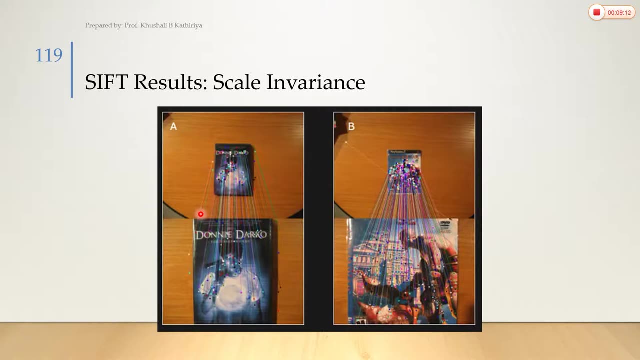 Intersection. That means its SIFT features. How much are they matching? Okay, So this one is the three comparison method for the SIFT features. Okay, Now, this one is the application or this one is the result of SIFT. 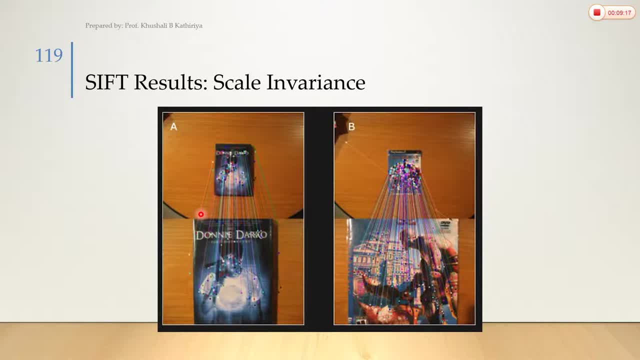 These SIFT features. First one is the scale invariant. We have seen scale transformation. What is a scale transformation? Scale transformation, that means zoom in and zoom out. Scale transformation, that means you have to resize your original image, That means you have to enlarge it. 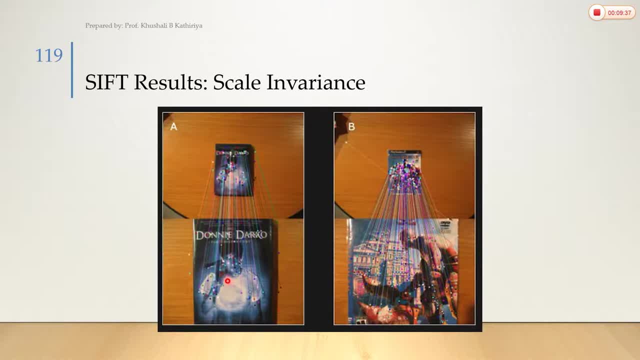 Okay, So suppose one is your image A and one is your image B. Here this one is small image and this one is scaled image. Okay, So here we have to check in these two that these two images are same If we manually check, like human eyes. 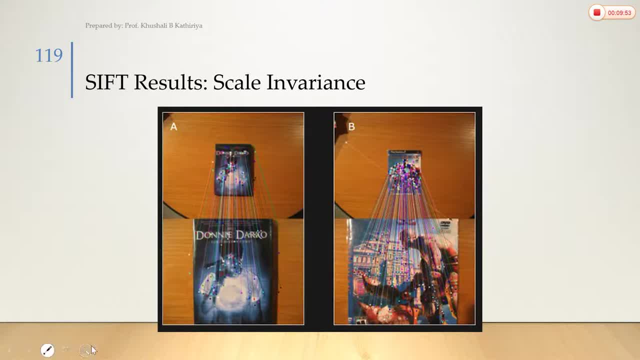 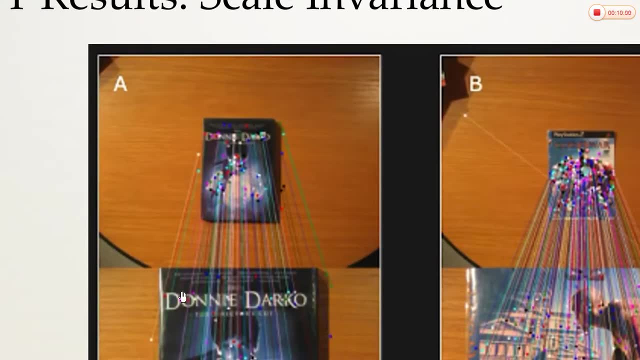 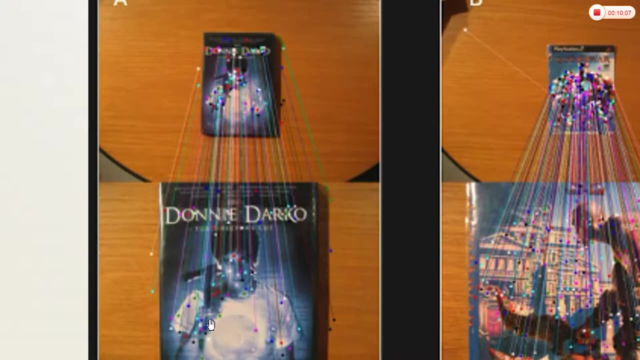 Okay, So see here something is written Here. it is not visible. If I use magnifier, then see, Something is written here. and same to same something is written here. Here is some picture of some boy. Same to same. here is a picture of some boy. 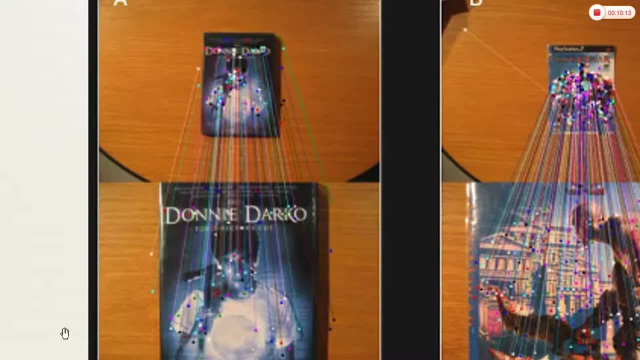 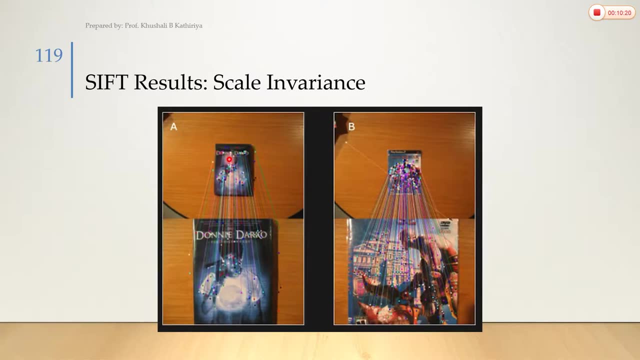 So we can see manually. We can check that. no, no, no. This one is This one. How do we do? We can check this. So what these two images are. this book is same, But how the computer will find out that these two are same. 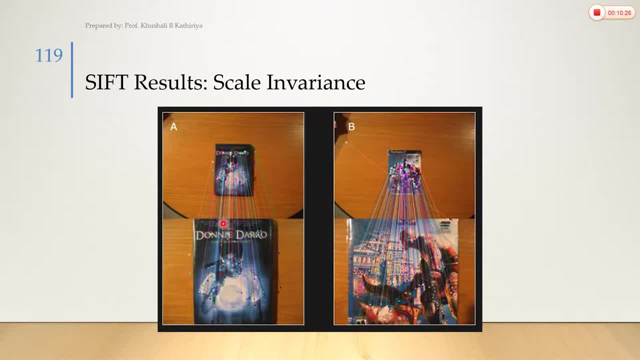 So what its done? These two features will be identified First of all. what it will do? It will identify its features and identify its features. After this, it will compare the features of both If the distance between the features of both comes to the minimum or 0 comes. 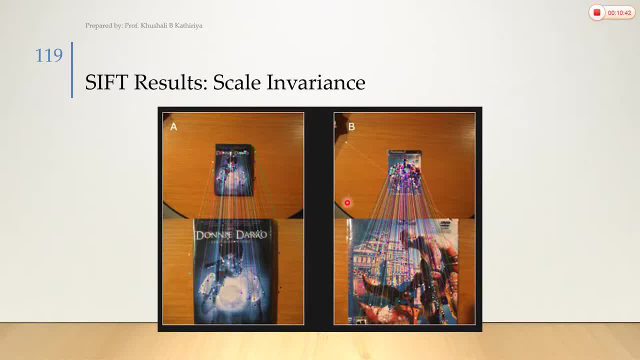 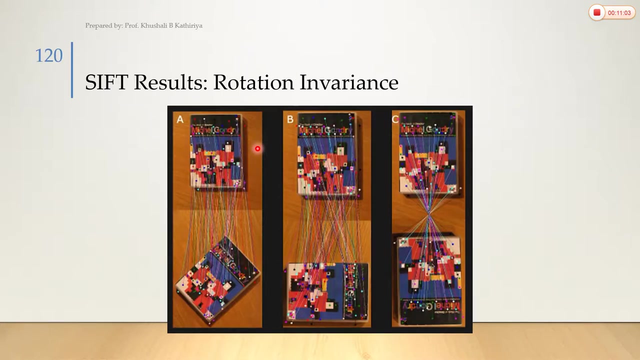 That means these two are the same, Same to same. for the B image. Okay, If we check manually then both are same image. So SIFT results are 100% sure about the scale invariance, Even if the scale is different. but SIFT results try to give 95-100% result. 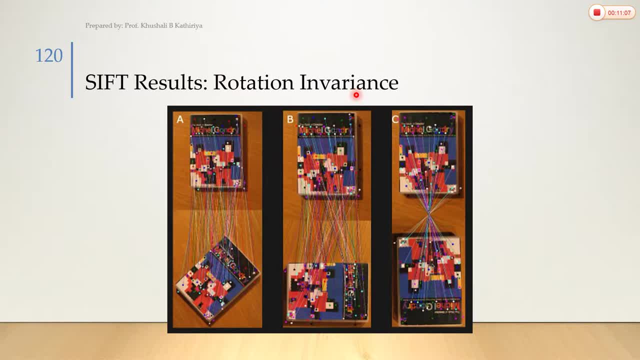 SIFT results for the rotation invariance. If your image is in rotated format, Suppose I have a book on 45 or 35 angle. This is the first book and this is the second book with some rotation. If I have to check both of them whether they are same or not. 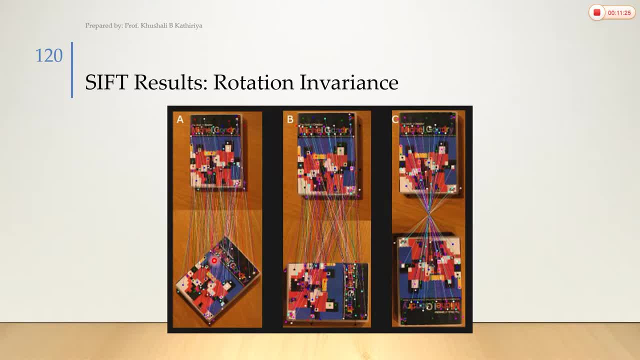 Then it will identify the features with this image. But it will successfully identify That means this one is 45,, this one is 90 angle and this one is 180 angle. So in all three images it successfully patch the result. That means SIFT results are successfully derived for the rotation invariance. 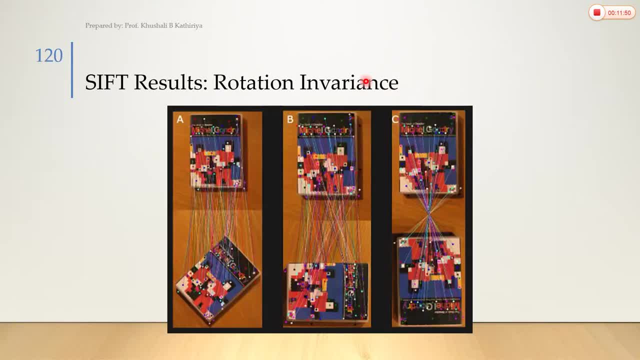 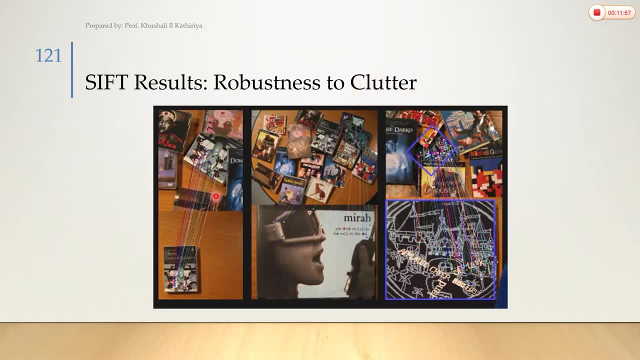 That means it gives the result for scale invariance. It also gives the positive result for rotation invariance, Robustness to the cluster. If you have a multiple area, multiple cluster and you have to do classification And you have to identify a book from that. 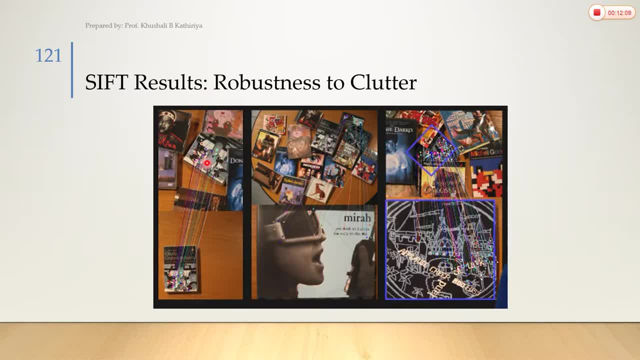 Then you have to give that book And you have to give that book. What you have to do above that book? What you have to do above that book, You have to identify a book from its cluster. That means this one is one book and this one is multiple book. 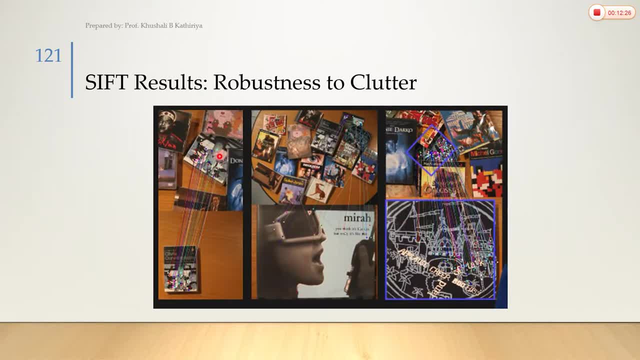 You have to identify all the features of that image And you have to compare all the features with this book. Whatever book will successfully match that book. That means this is its feature. its SIFT result is printed. Okay, same to same for this. Here is this portion. what has it done by zooming here? 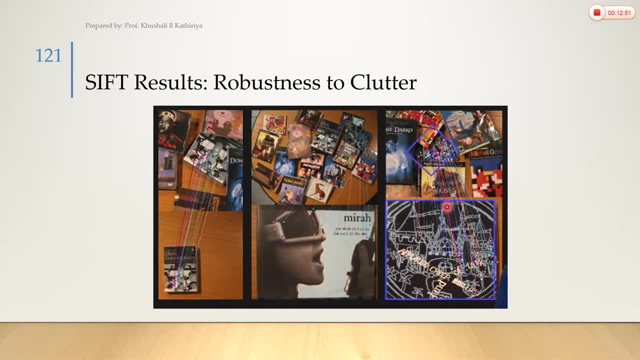 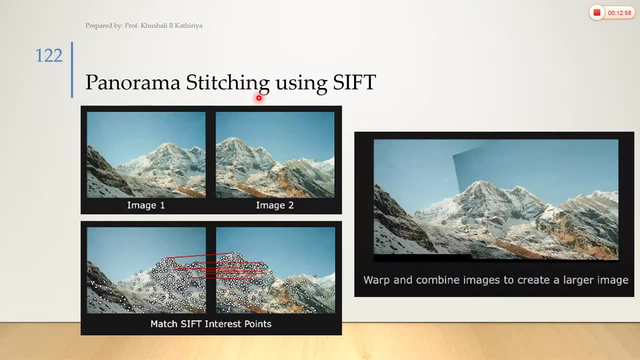 It has been shown by comparing Same to same for this book. Okay, so it has also been shown by zooming here. So this is the concept and this is the example for the robustness to the cluster. Now they will also use SIFT result for the panorama. 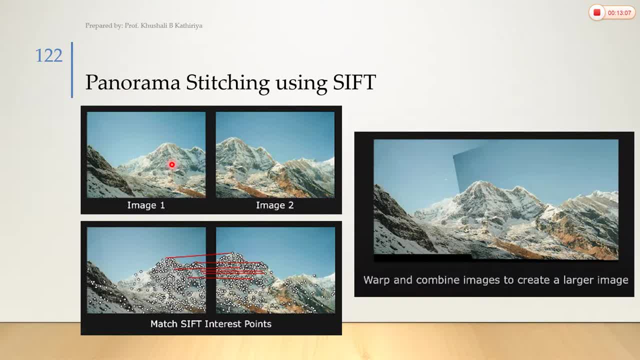 Panorama. that means you have two different images. they have been clicked at the same angle and both are of the same object or of the same environment or of the same place. If you see these two images here, then this portion is being repeated here. 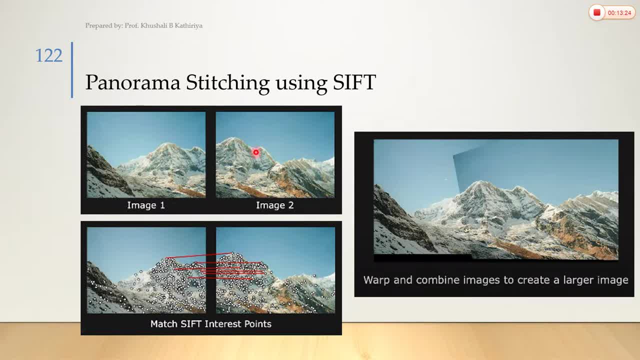 Okay, this portion from here to here. But what we have to do, we have to merge this portion that is being repeated and make all the images one image. That means we have two different images. what we have to do with those two different images? 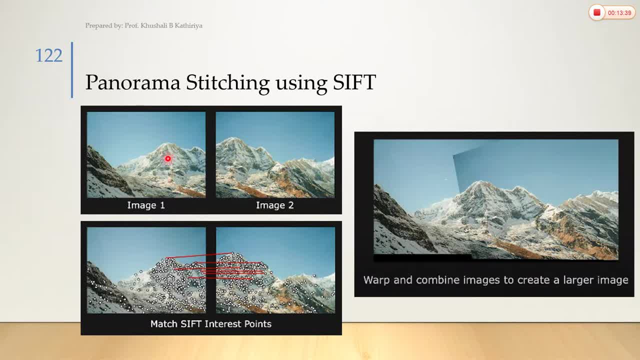 By merging, one image is made. So what we have to do here, We will identify the SIFT features of this image and we will identify the SIFT features of this image. What will we do with the features that are matching? What will we do with the interested point? 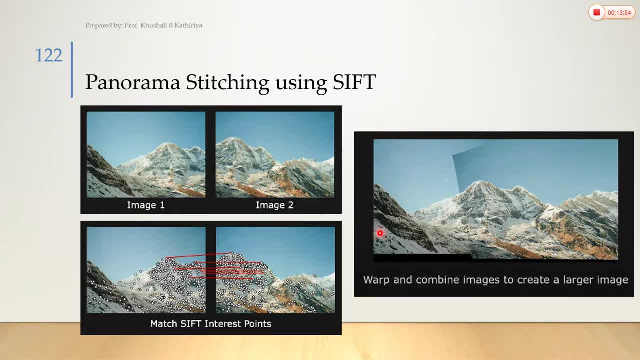 We will match it. And after that, what will happen? We will merge it, We will combine it, Wrap and combine the images to create the larger image. So see here what happened to both the images. They have been matched. If we see these two from here, 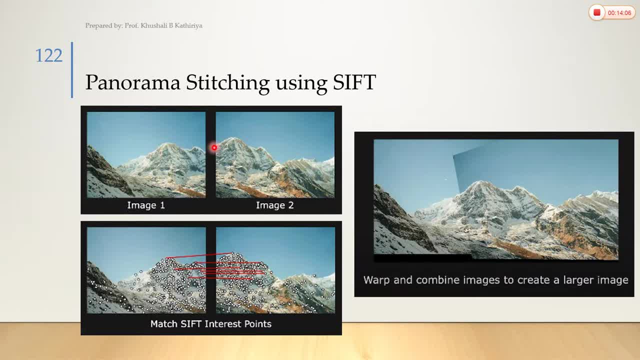 then something is being cut from here. They are being started again from here. So what happened From here to here? the image will be combined. That means we have received a larger image from compared to another two images. So this one is the example for the Pornorama Stitching using SIFT. 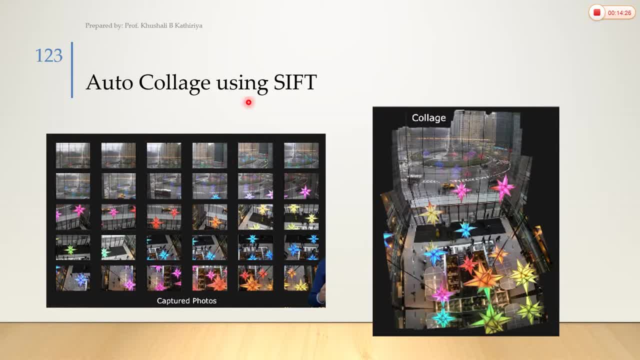 Also used for the Autocollage using SIFT. If you have multiple images and you want to make a collage of them, then what you will do, You will combine them. So by combining, we can make a collage using SIFT. 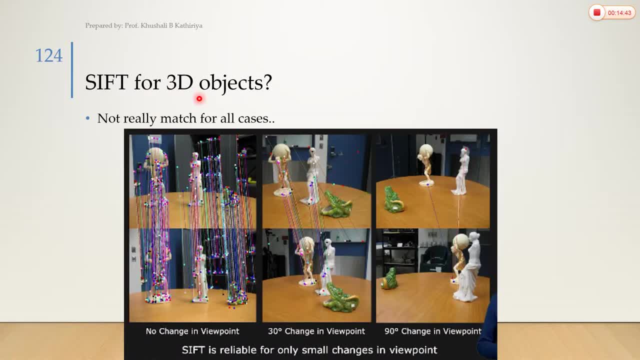 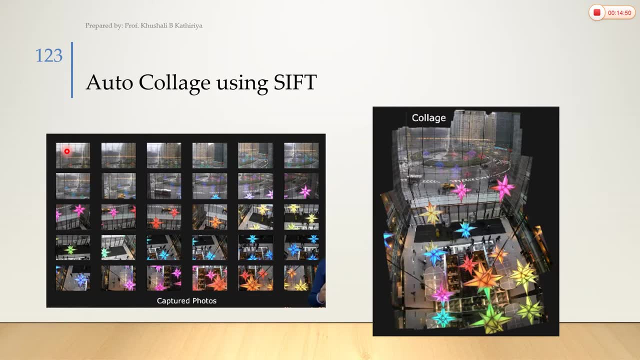 And the last one is the SIFT are used for the 3D object. 3D object that means what will happen in 2D object. In 2D object you can change the angle of the image. You can scale it. 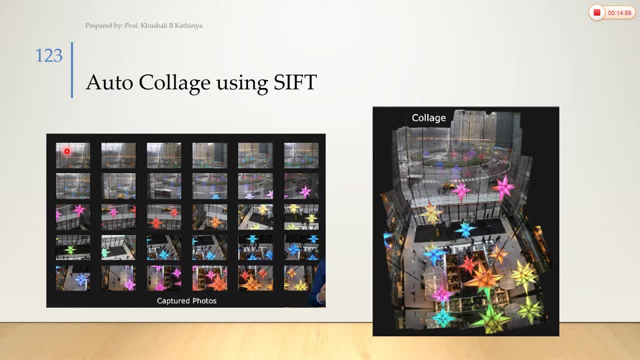 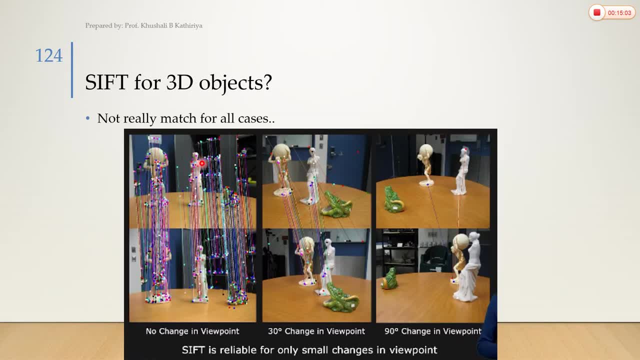 You can rotate it, But its view- suppose its front view- is there, you cannot do the back view. Okay. So if this is the image, See this image, The image here and the image here. It is clicked from the same angle. 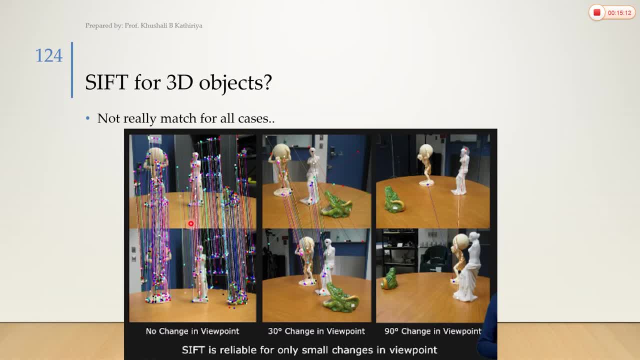 That means our view point is the same. So here no SIFT features fail. Okay, So no changes in view point. So that's why we have successfully matched our all features with A and B image. But see, here Some angle has been changed. 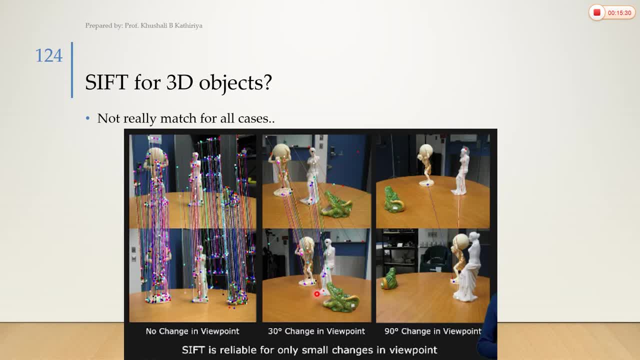 Okay, Here is one image here, And one image has come a little further And here some angle has been taken from the back. Okay, I can't say further, But here it has been taken from the back, It has been clicked. 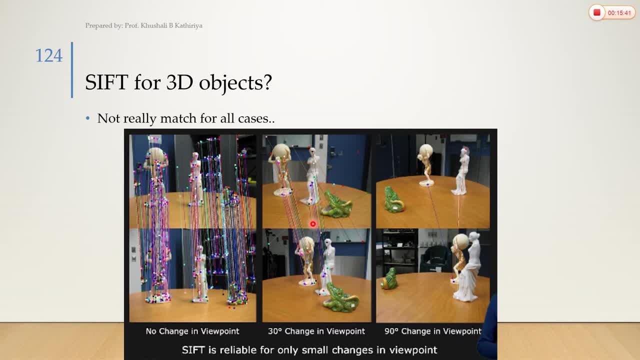 And after that, what has it done? It has clicked. So what is happening with some of its features? It is being mismatched. See here, This portion, This portion, This portion. Here also what is happening with some features. 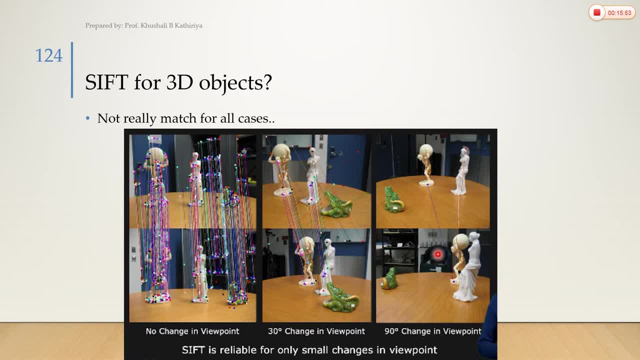 It is being mismatched Same to same. If we have the angle of our image, we can change it at 90 angle. That means this one is the front And this one is the side view. So what will happen with its SIFT feature? 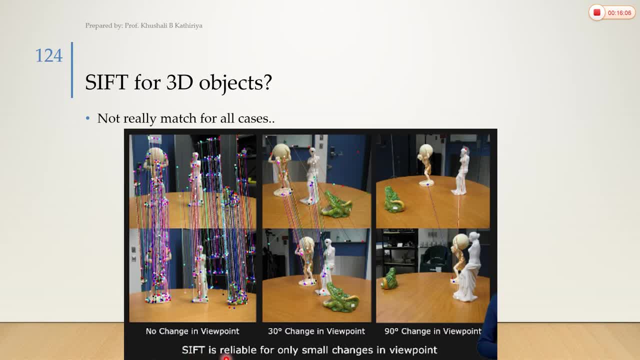 It will be extremely changed. That means SIFT is reliable for the only small changes in viewpoint. If there are small changes in our viewpoint, that means it will match to some extent, But if it is too much, its viewpoint is different, or then we have changed our angle. 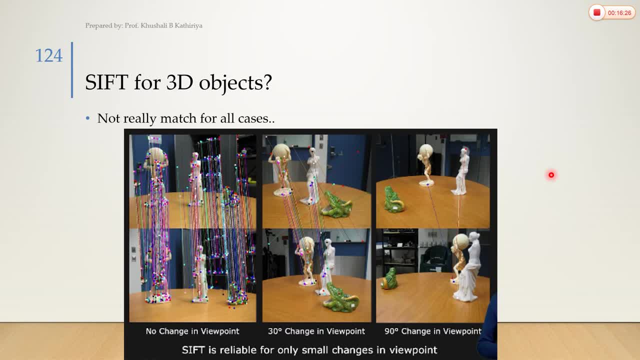 Suppose this one is our front side. Suppose you have a Dean, Okay, Pepsi is written on the Dean. If Pepsi with another Dean, we will compare both of them. Both have front. If Pepsi is written, then what will happen? SIFT features will be the same.